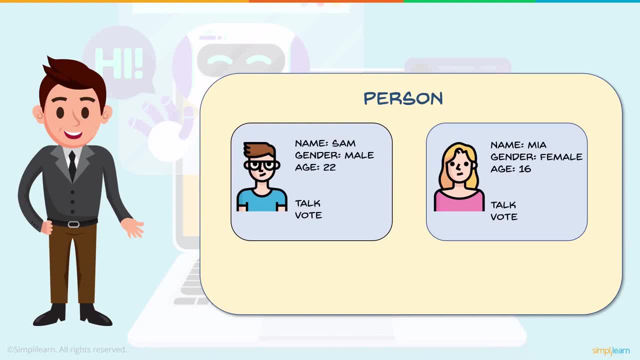 these two objects, two separate entities, then It's the value of the features. So our features- name, gender, age- in either case has a different value. For example, our first object has the name Sam. Our second object has the name Mia, Our. 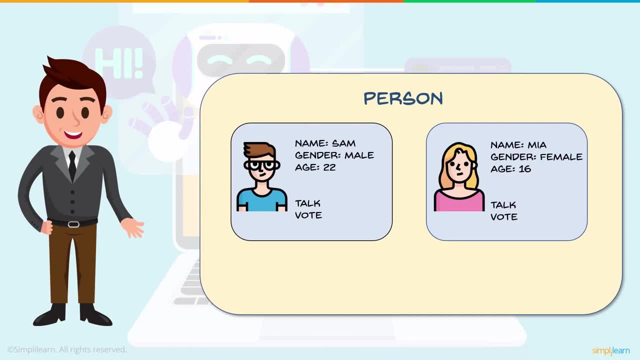 gender is male and for a second object, gender is female. Age is also a different value for both our objects. Now they could have the same value, that is, there could be some common features, but if all of them have the same value, that wouldn't make sense. They wouldn't make them two separate objects. So to 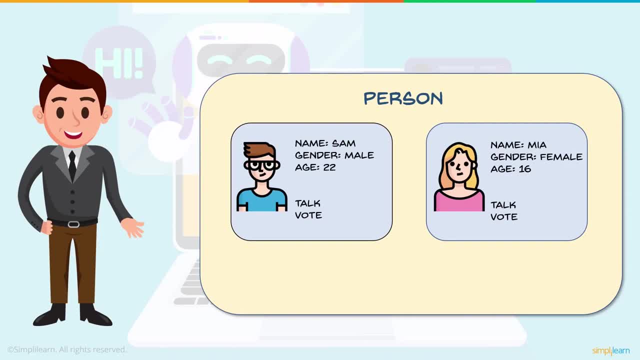 summarize: this person is a class and the class defines the features: name, gender and age. It defines behaviors- talk and vote- and we defined two separate objects and gave value to the features in these objects. Now let's begin to code this example. So I'll move on to PyCharm. First thing first. 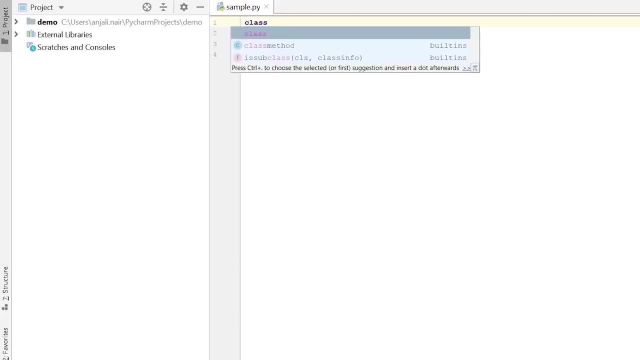 let's create our class. So our class is created using the keyword class, and then put down the name of your class, which in our case is person, followed by colon, and enter, So your class is created. Now, once that your class is created, the next. 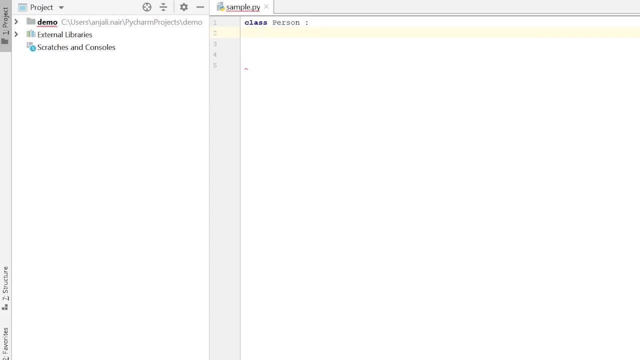 thing we need to focus on are the features that this class defines. So the person class defines the features name, age and gender. Now, in our previous video on oops, we saw that the features or the members of a class are defined using a constructor usually. So let's create a constructor. 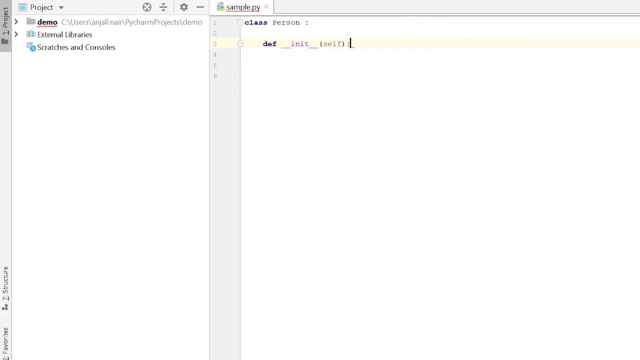 which is def init, and once you click on init, the self parameter automatically appears. Self basically refers to the object that you're passing to this constructor or the object that is being created when the constructor is called. Now we'll give value to our three features. So features are name and that. 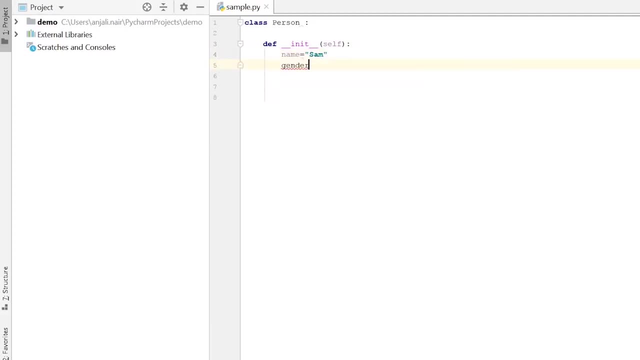 will have the value, say, Sam, gender, male and age 22.. Now, one thing that we are missing out here is that we need to remember that name. gender, age- all these are features of the class. That means these features are strictly tied to an object. That would be the object that's created when this init function. 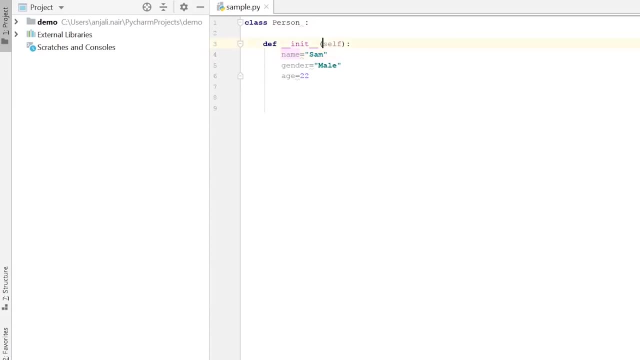 is called for that particular time. So the reference to that object would be stored in self. Therefore we won't just write name equal to Sam, but instead self dot name equal to Sam and in a similar manner, self dot gender and self dot age. So we have defined our features. 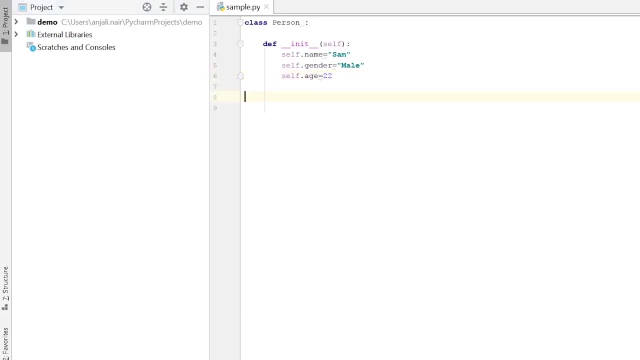 of the class person and also given it value. Now next thing is you have to define the behaviors. So behaviors are implemented through functions, or we can say methods. So methods are basically functions, but the functions which are called through an object or tied to an object are called methods. So let's 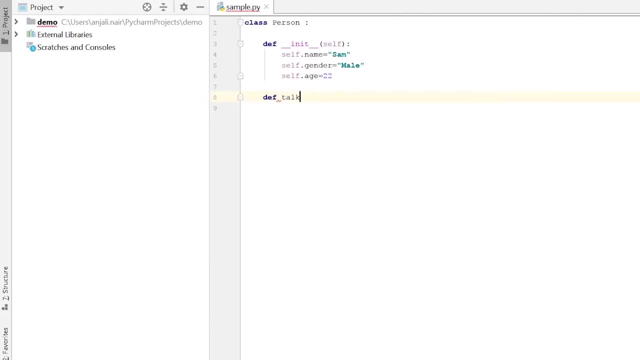 define our methods. Our first behavior is the talk behavior. So if the talk method is called, we just want to print out hi, I am and the value of the name, attribute of the name, the object that's calling talk. now our next behavior to be implemented is the 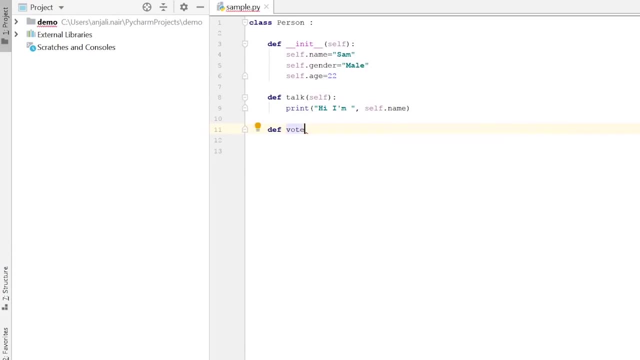 vote behavior. so for that we'll create a method vote and here we'll put in a condition. so if the age of the person is less than 18, the person's not eligible to vote. so we'll print this out, and if the person is above 18, then we'll print. 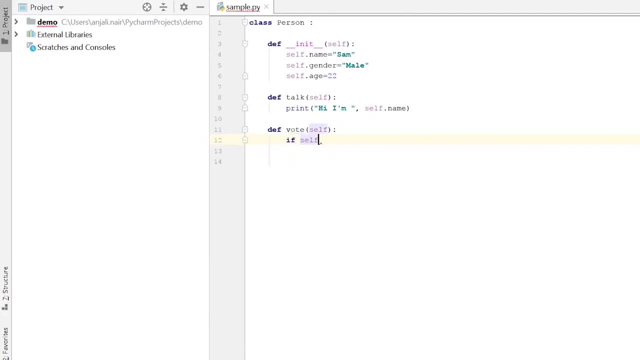 out that the person is eligible to vote. so if self dot age is less than equal to 18, I am not eligible to vote, actually less than 18. if the person is 18, they are eligible to vote and sprint I am eligible to vote. so the two behaviors of 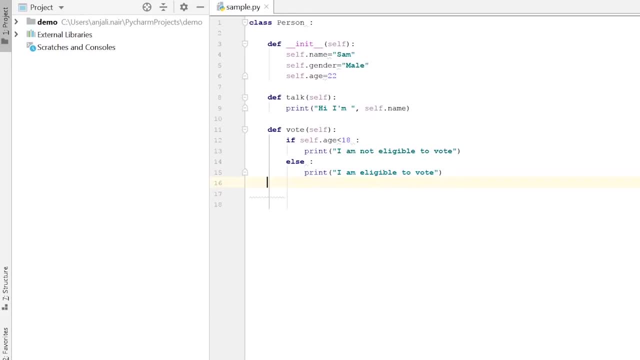 the class person' are implemented through methods. now. Now, all that's left for us to do is to create the actual object. So how do you create the object? If my object name is obj, I'll write obj, equal to, and then put in the type of the object and the type. 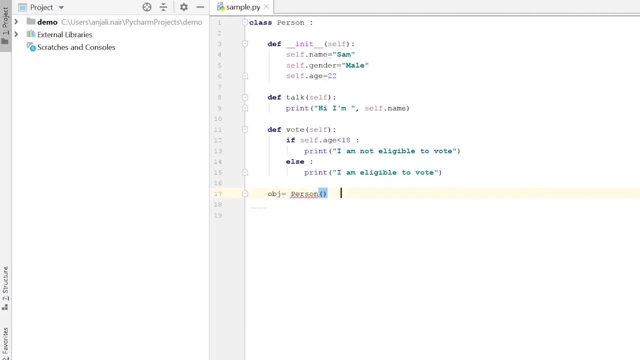 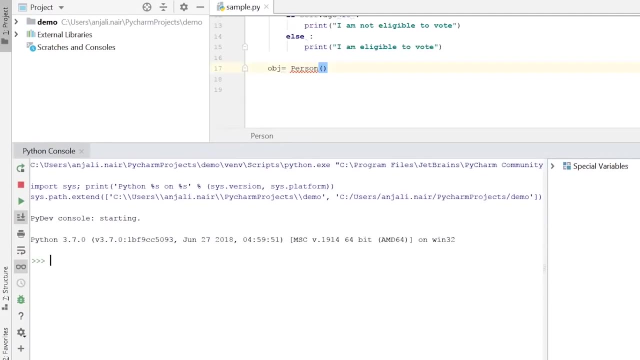 of our object is, of course, the class. Now here's something that you need to understand: Everything that you create in Python is actually an object, So I'll explain this a little more in my console. So if I have a variable, say a, and I give 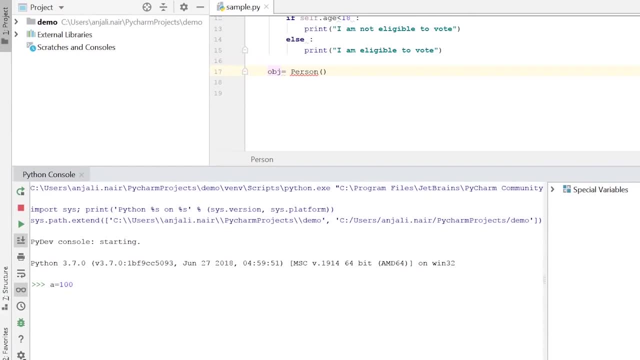 this variable the value hundred. We know that hundred is an integer type value. therefore that makes a an integer type variable. But then if I check the type of this variable, it shows class int. That means the type of a is the integer class which makes a an object. In the similar manner, if I have another value to a say, 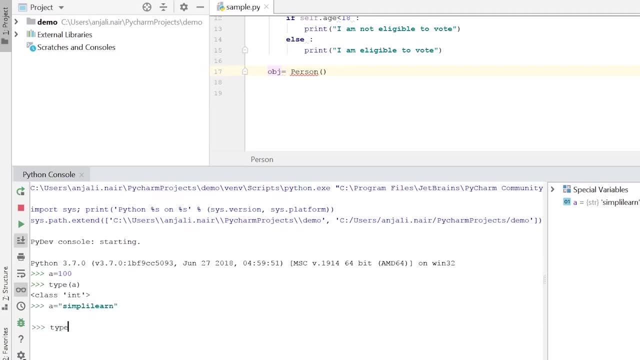 simply less. it means class int. and now, if I check the type of a, we'll see that a is now an object of class string. STR is basically the short form of string. therefore, everything in Python is an object of some class, and that is how our object here, obj, is an object of. 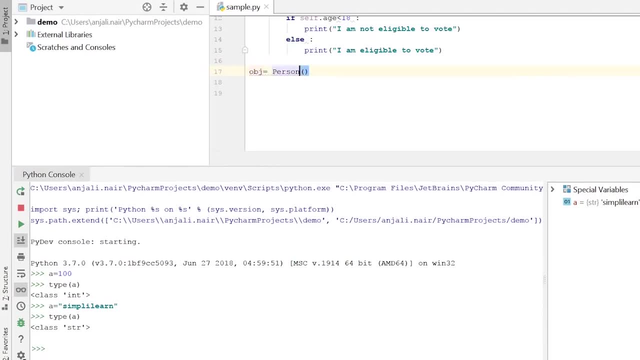 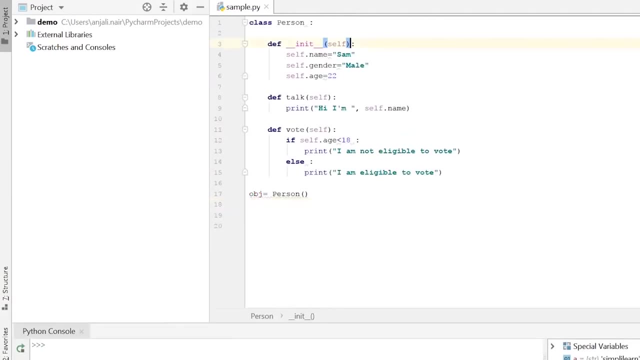 the type person, where person is our class. so now that we have created an object, during this creation of the object, our constructor will be called and the features of this object will be given some value. now we can use this object to call its behaviors. so this can be done either in this manner. so you put: 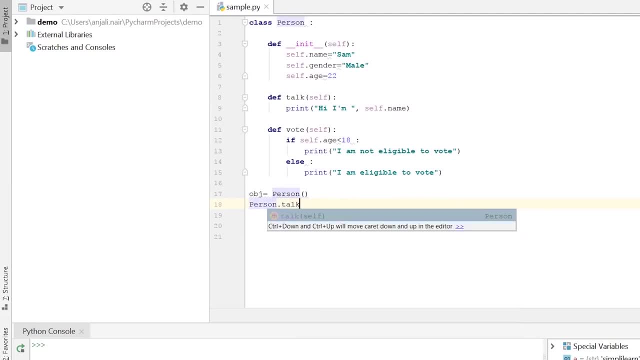 in person, which is the type of our object. dot the method and within the bracket, as a parameter, you can pass the object in the similar manner. we'll also call our behavior, vote and again pass obj within it. now let's run this code. just pull up my computer. 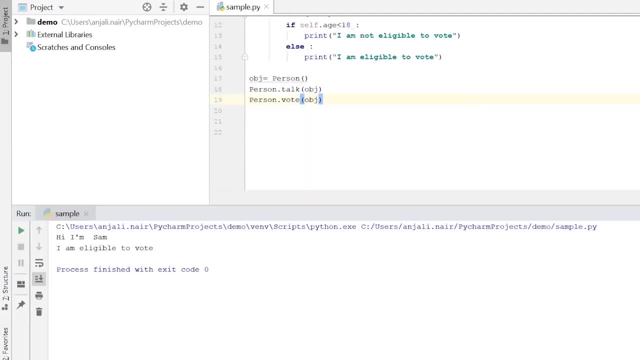 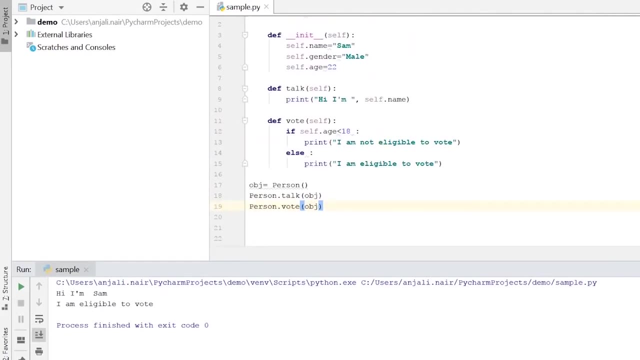 so here run the program and as you can see here, so we created an object and the object got its values as mentioned in the constructor that is in it, and then we call the talk behavior or the talk method, using our object obj, and this printed our first line, which is: hi, I am Sam. and then we call the vote behavior. 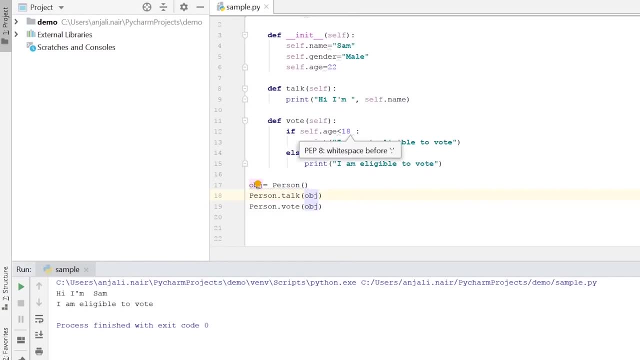 and in the vote behavior, the age of our object was checked. since our objects age was greater than 18, it says I'm eligible to vote. now these two lines where we are calling our methods can be done in a different way. instead of calling it with the type of our object and then passing our object, we can directly call it with: 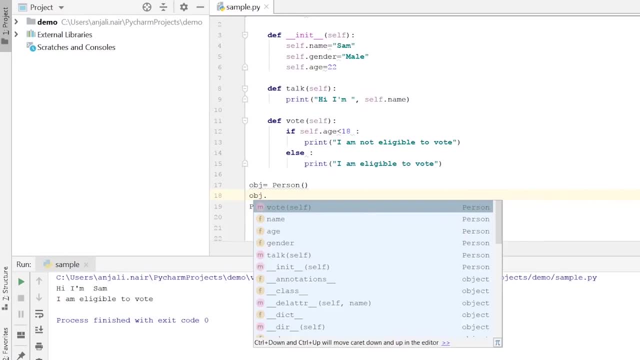 our object. so we can have it in this way: obj dot talk off, and over here obj dot vote off. so we must remember that in this particular case, where we are creating classes and objects and have this kind of a structure, all these methods are actually tied to the object, which is why we cannot just say talk off, we need an. 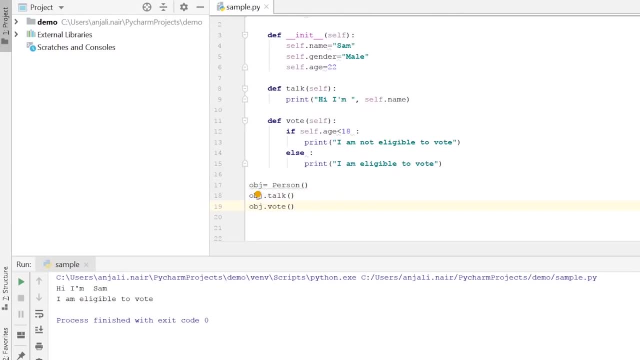 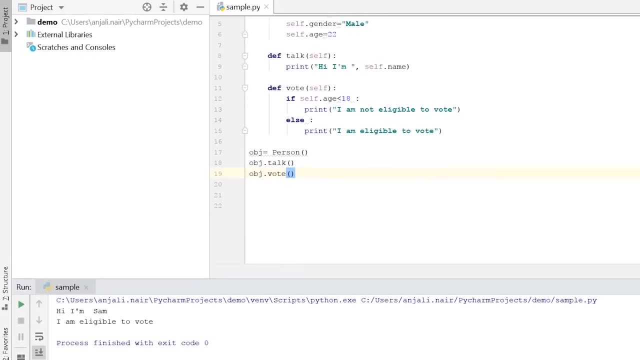 object, to call it or at least pass an object to this method. let's run the code now, so it's the exact same result works just fine. now, in this case, we just created one object and the values for this object were predetermined and just put in our constructor. now what if we want to create two separate objects and 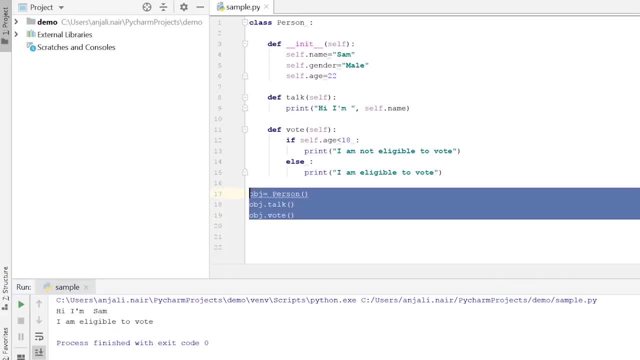 the values for these objects vary. so in this case, so to demonstrate this, we'll create two objects, just like in our example previously. we'll have our first object, which is obj one. now, both these objects will be, of course, of the type person which is our class. so put that there now. every time the 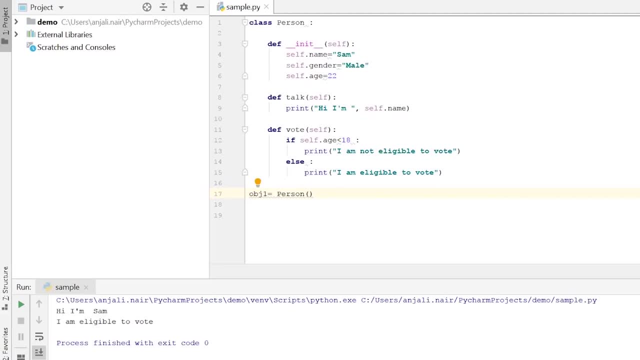 object is created automatically, our init method is called. so if our object needs to have separate values, what we can do is, instead of putting in predetermined values here, we can pass the values for the features of the object in the brackets. so if I want my name to be Sam, I pass Sam, my gender and the age. so 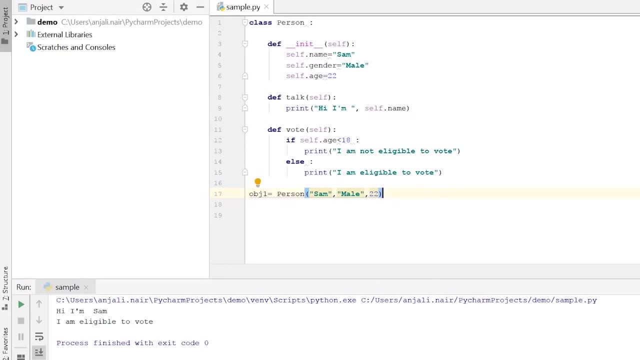 these are the three values for the three features that this object has, which we will pass into the constructor or the init method. now, in the in it method, we need to be able to accept these values. so, other than self, we have one variable which will store the value. 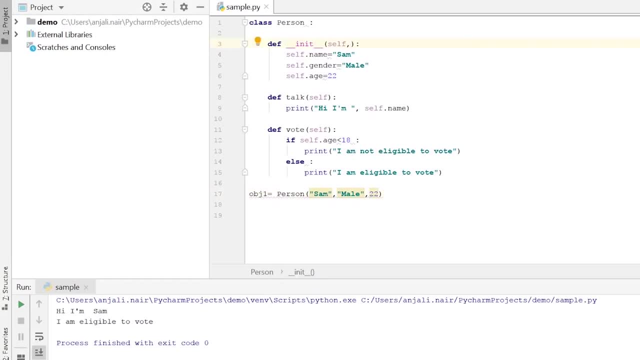 the name when it's passed from here, We'll store it in variable n- n for name and the gender, we'll store it in variable g. age: we'll store in variable a. So what happens here is basically: these values that you pass within the parenthesis when you're creating your object are sent to your init method. 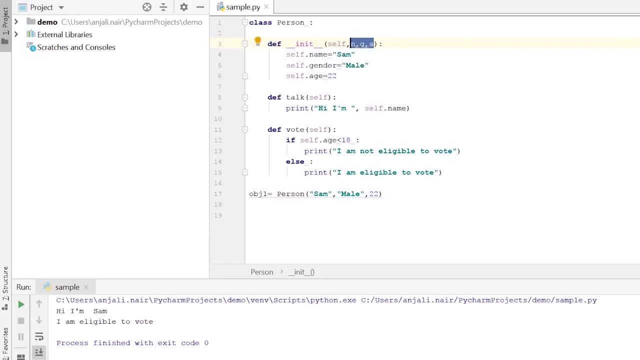 Now in the init method we are putting down these three variables to accept the values. So these three variables store these three values. So sam goes to n, male goes to g and 22 goes into a. Now, instead of putting in the strings here, selfname can be equal to n, So the value which 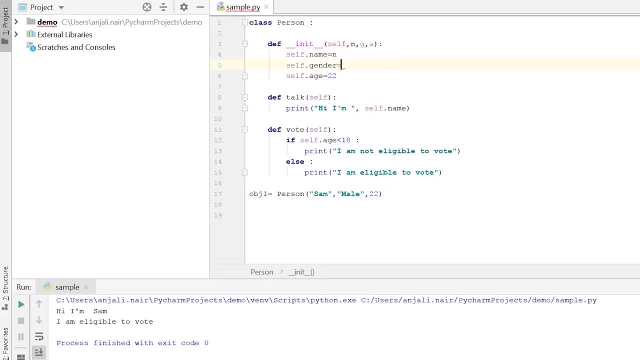 n got is now put into selfname, and the value which g received is put into selfgender, and the value which a received will be put into selfage. So that way we created our object and provided a way in which we can actually have unique values for each object. 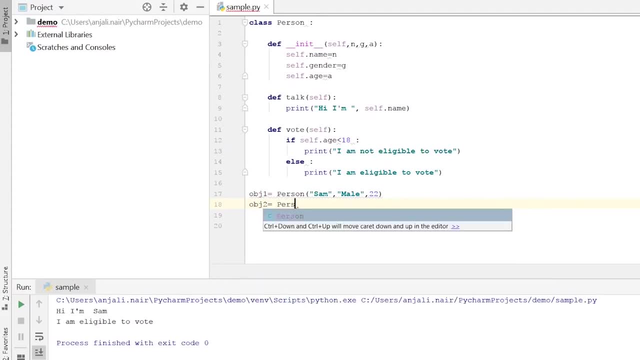 So now, if we have another object, say obj2, which is also of the type person, we can put in different values into these parenthesis. So say, our second object's name is jessie, She's female and 16 years old. So now these values will go into these variables and will be assigned to these features. 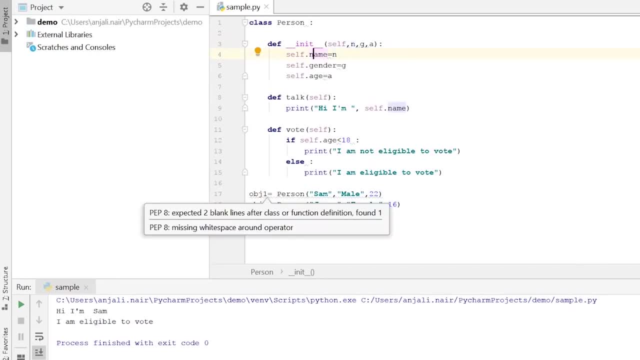 So for obj2, obj1, if I say obj1.name, the name would be sam. If I say obj2.name, it would result in jessie. We'll see that now. Let me just print that out: obj1.name and obj2.name. So as you see. 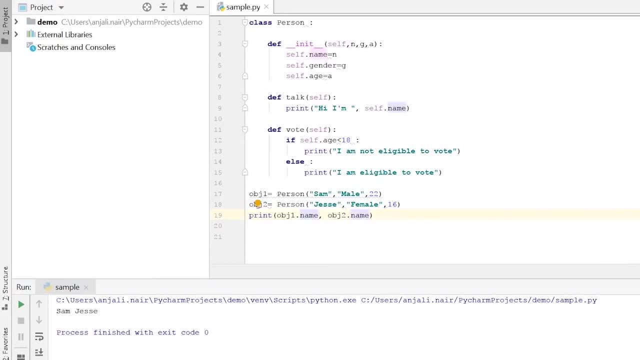 although our feature is the same, we are printing the feature name. in both the cases, the object to which this feature is tied is different. So the first time it's printing name related to objectname, Object 1, and the second time it's printing the name related to object 2.. Now, this is not what we. 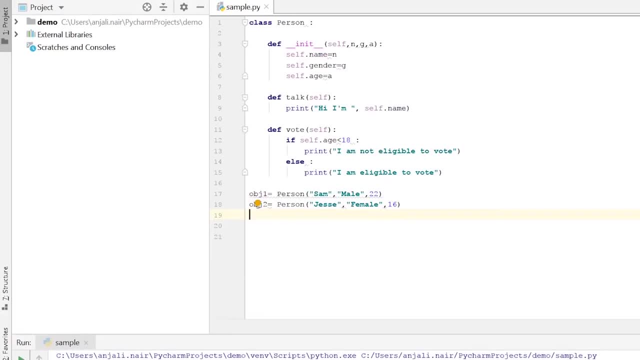 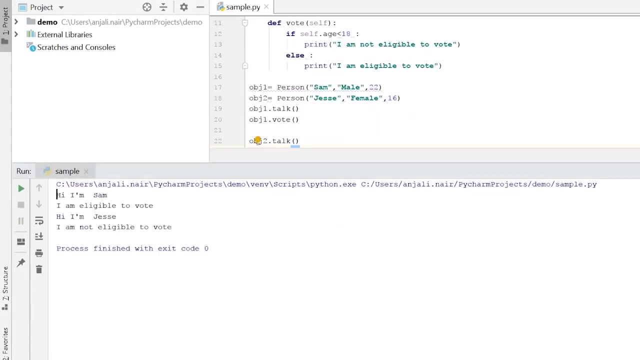 want to show here. Here what we want to do is, after creating our two objects, we'll call the methods using these objects, So obj1.talkOf and obj1.voteOf. Now we'll call the same two methods using obj2.. So obj2.talkOf and obj2.voteOf Run the program and here's our output. 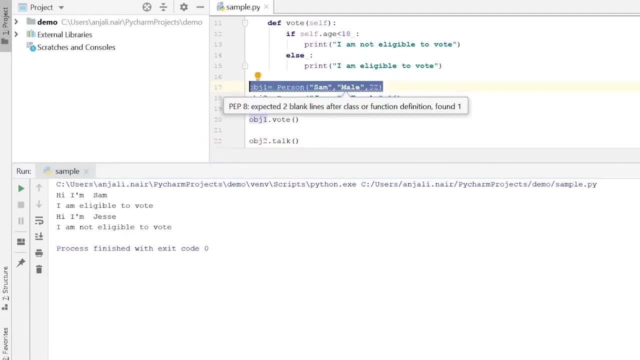 So what happened here is: obj1 was created and the three features, which are name, gender and age, were given the respective values for obj1 and, the similar manner, obj2 also received the values for its various features. Now we used obj1 to call our two methods: talk and vote At talk. all we did is 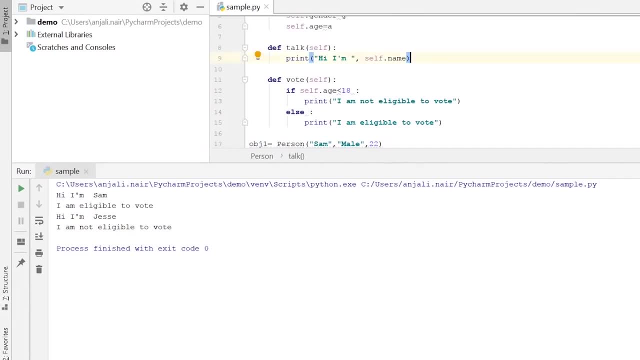 print our name of the object. So the first time when we called with obj1 it printed hi, I am sam, first object and then we call the vote method using obj1 itself. So our first object's age was 22, which means it's eligible to vote, and that is what's printed here: I am eligible to vote.